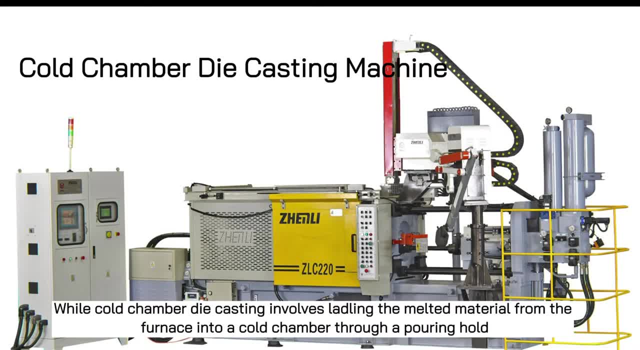 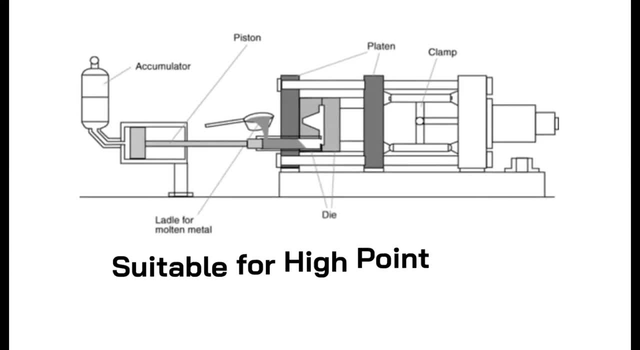 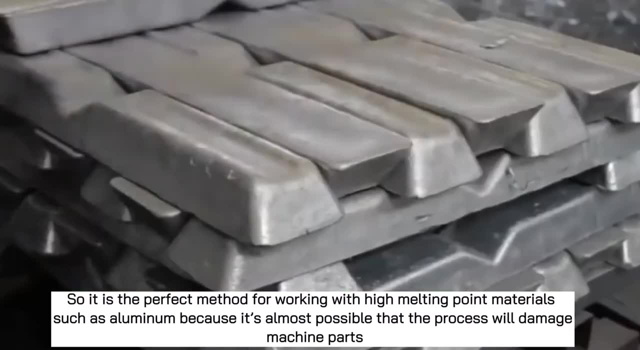 While cold chamber dicasting involves laddling the melted material From the furnace into a cold chamber through a pouring hole. What's more, cold chamber machine works with horizontal position and don't include a gooseneck, So it is the perfect method for working with high melting point materials such as aluminum, because it's almost possible that the process will damage machine parts. 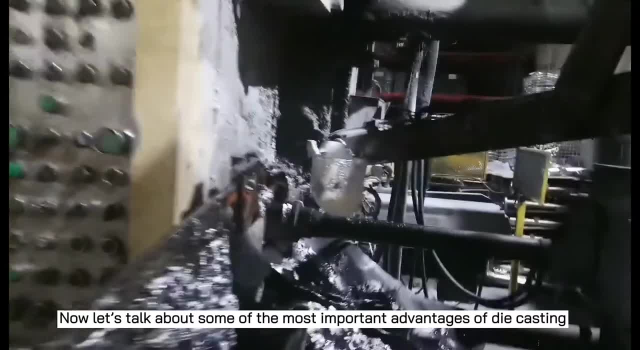 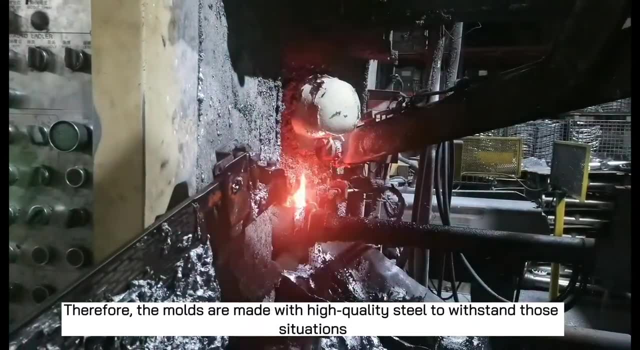 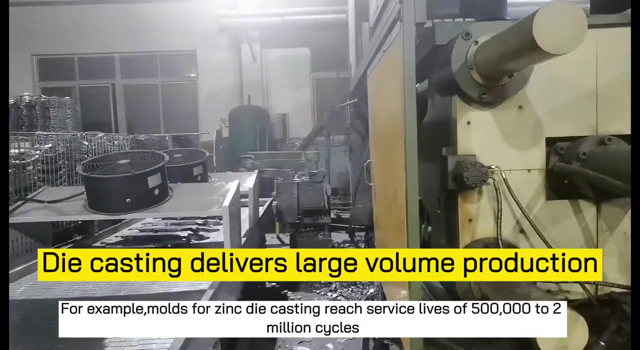 Now let's talk about some of the most important advantages of dicasting. The dicasting process exposes the tools to extreme thermal and mechanical pressure conditions. Therefore, The molds are made with high quality steel to withstand those situations. For example, molds for zinc dicasting reach surface lives of 500,000 to 2 million circles. 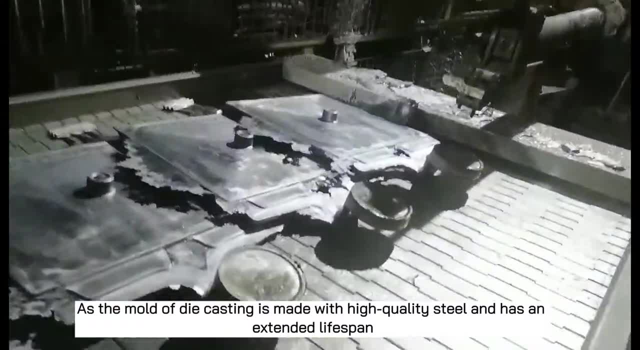 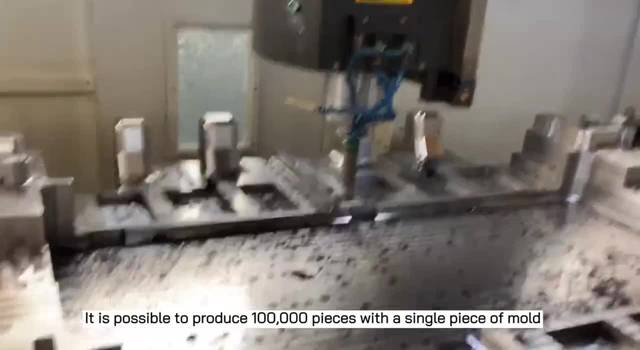 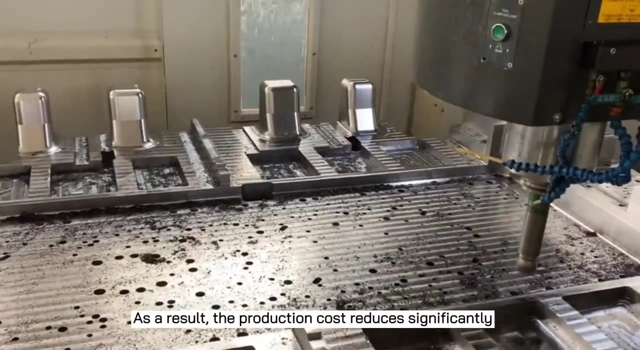 As the mold of dicasting is made with high quality steel and has an extended lifespan, they are capable of producing a huge amount of cards in a short time. It is possible to produce 100,000 pieces with a single piece of mold. As a result, the production cost reduces significantly. 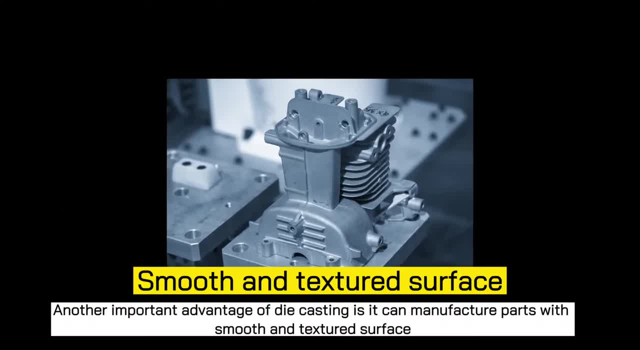 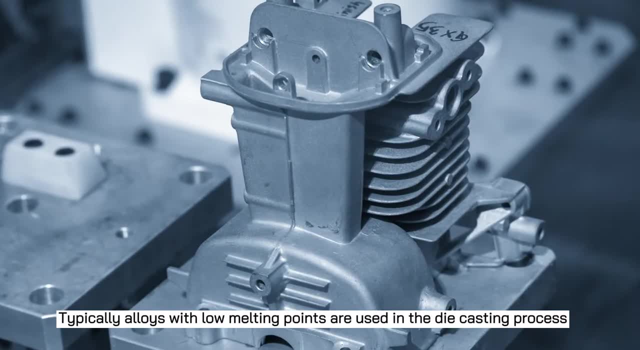 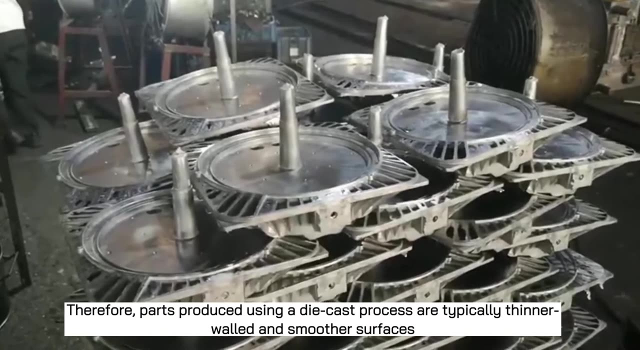 Another important advantage of dicasting is that it can manufacture parts with smooth and textured surface. Typically, alloys with low melting points are used in the dicasting process. Therefore, parts produced using dicasting process are typically thinner-walled and smoother surfaces. It also makes applying further surface finishing easier. 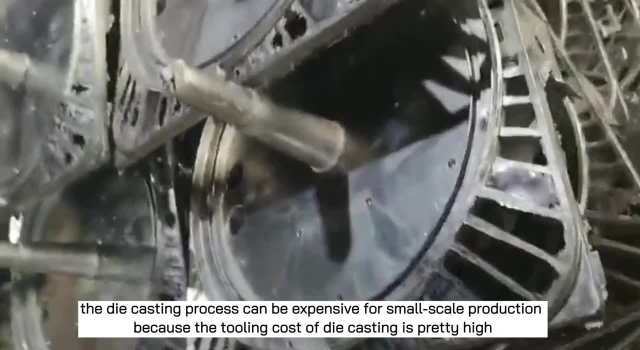 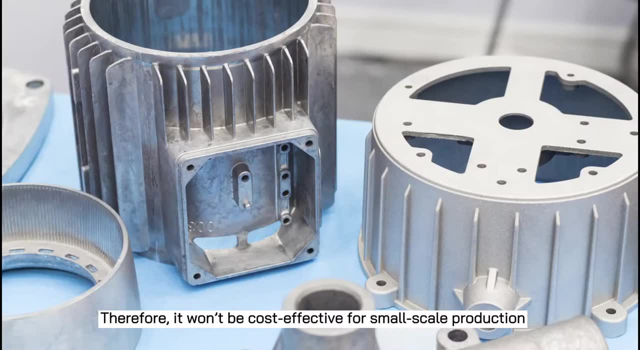 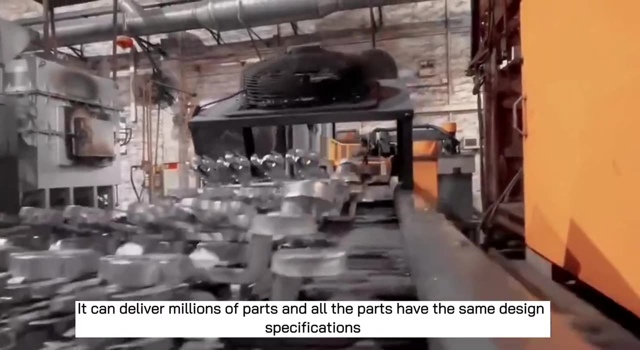 However, the dicasting process can be expensive for small-scale production because the tooling cost of dicasting is pretty high. Therefore, It won't be cost-effective for small-scale production. Dicasting is a blessing to the manufacturing industry. It can deliver millions of parts and all the parts have the same design specifications. 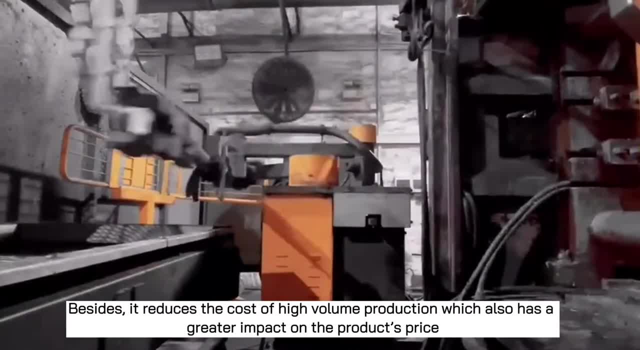 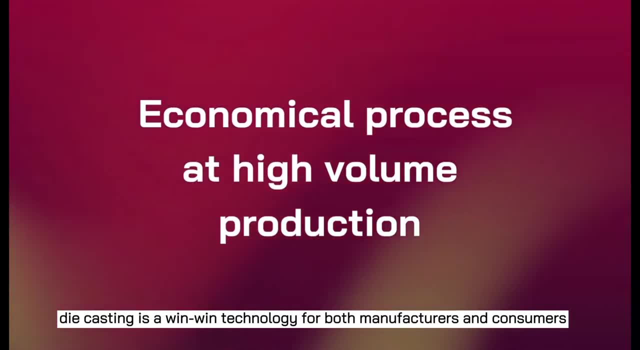 Besides, it reduces the cost of high-volume production, which also has a greater impact on the product's price. Finally, we can say dicasting is a win-win technology for both manufacturers and consumers. If you want to learn more or have any project in your mind, please get in touch with us. 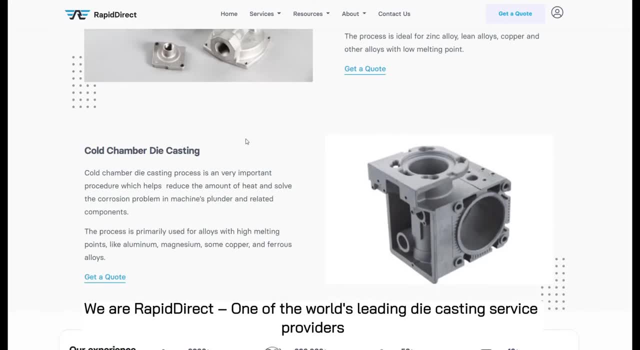 We are Rapid Direct, one of the world's leading dicasting service providers, And don't forget to like this video and subscribe to our channel to see more similar videos.